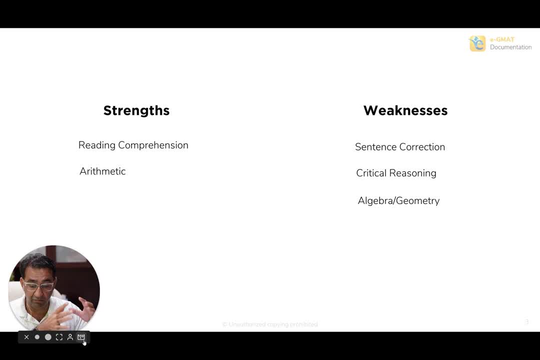 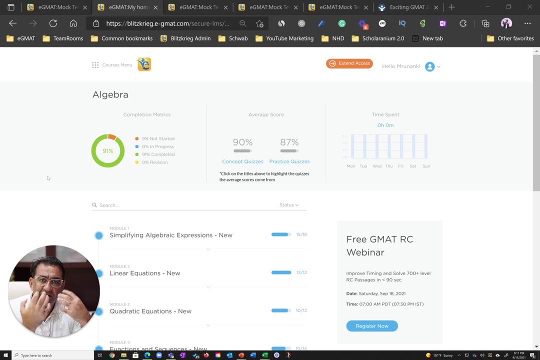 started working on quant first, and he started working on algebra and geometry first and next. I'm gonna walk you through how he turned this weakness into his strengths. Probably the most important trait that you need to excel on the GMAT is diligence, and Runang displayed. 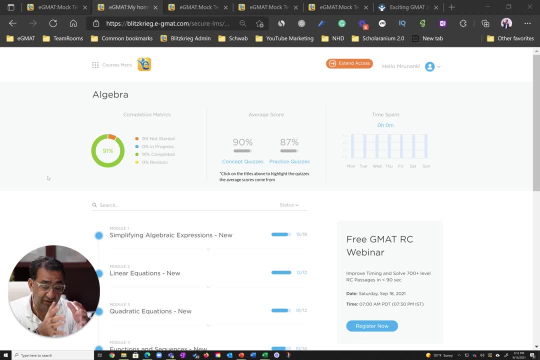 his diligence in the very first course that he attempted. This is the algebra course on the eGMAT platform. That's about 80 learning activities. Runang did most of the course. Not only that, he did it really well. Each learning activity within this course is evaluated, which means you get. 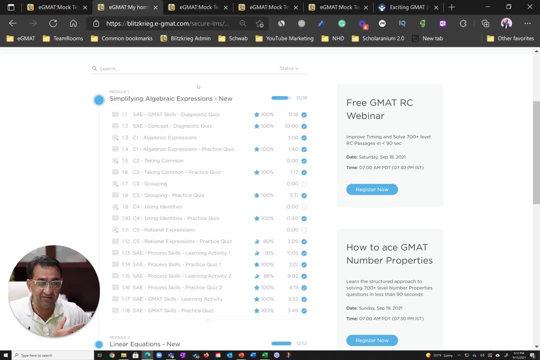 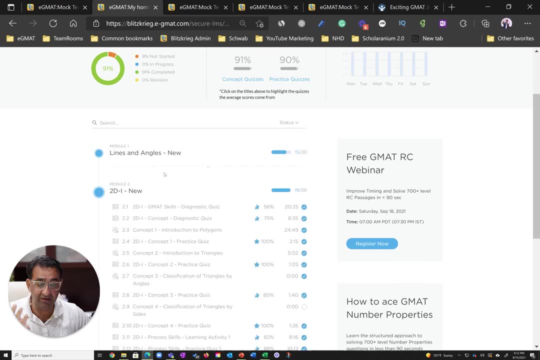 a score. Our expert AI guide tells you how well you've done and you can see he has really good scores or so. Similarly, in geometry, he invented Xhe repeated this feat. Now, geometry is a particular area of weakness for him. you can see how in. 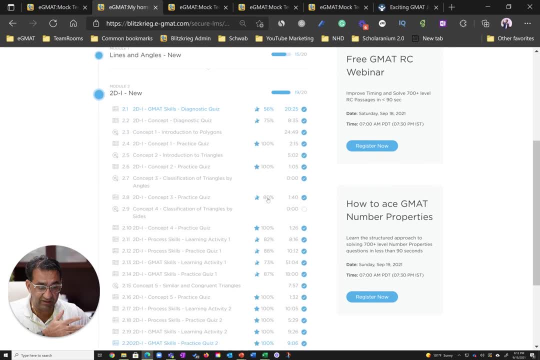 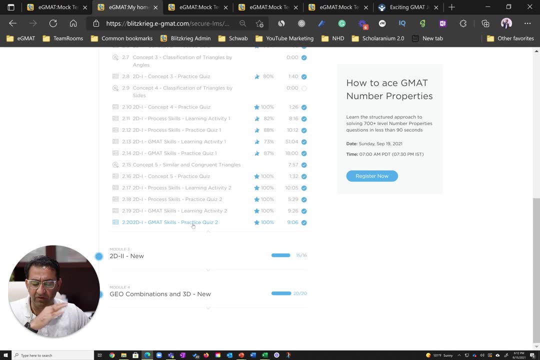 2D1, he had a very low GMAT skills diagnostics score, But then by the end of the module he was able to perfect this. Now, the thing to note over here was that he was able to do this all quickly: Runang tested in two days, And then he completed this course in two weeks. 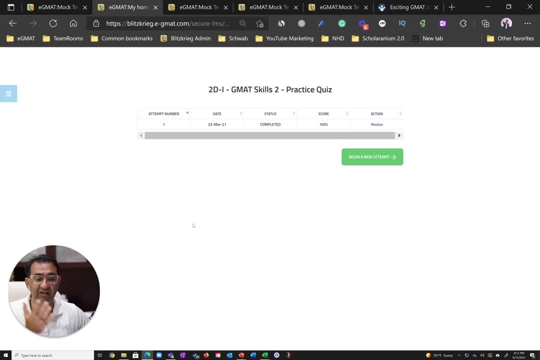 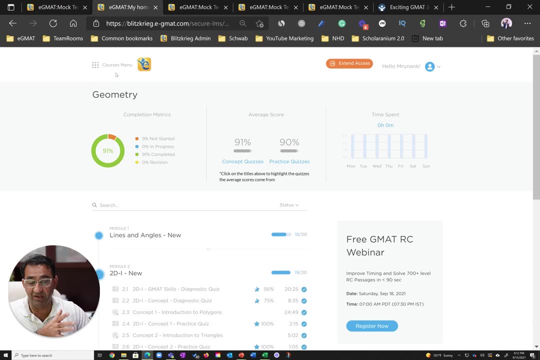 do this in the first go. As you can see, he only attempted this file one, and this was towards the end of March. Now, once Ronan was done with geometry and algebra, he moved on to sentence correction, And again he repeated this feat Again, as I say, one of the key traits of anyone. 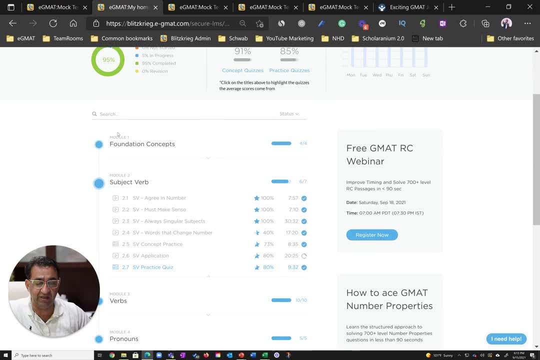 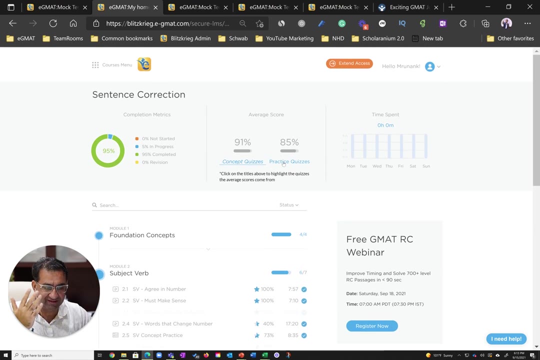 who wants to ASG matters is diligence, and he was really diligent. Now, mind you, there was a three week break when he was doing sentence correction. He actually suffered from COVID, yet this did not deter his diligence. He was still able to get really good scores in concept files- excellent. 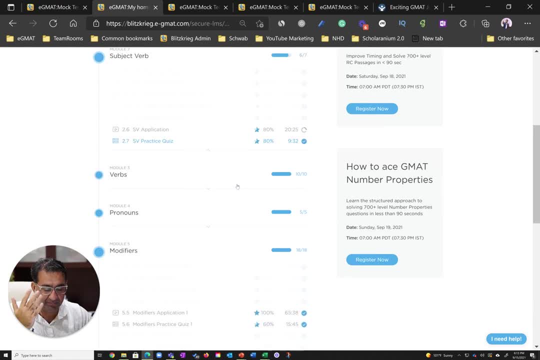 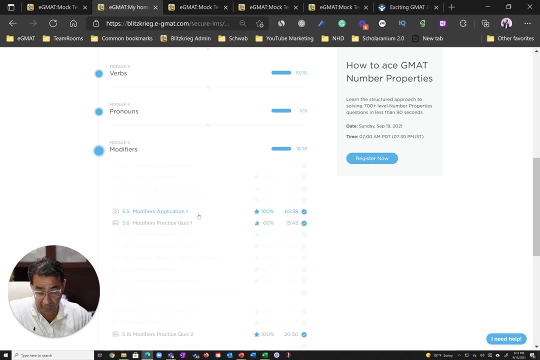 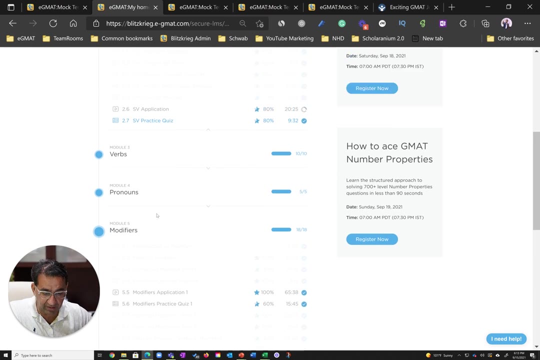 scores in practice quizzes And, as you can see, in certain cases I've only selected the practice quizzes. He spent considerable time on files when expert gave him feedback. The 65 minutes spent on application file one is a clear indication of the same. 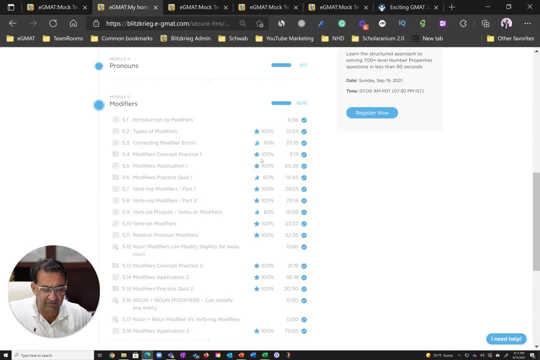 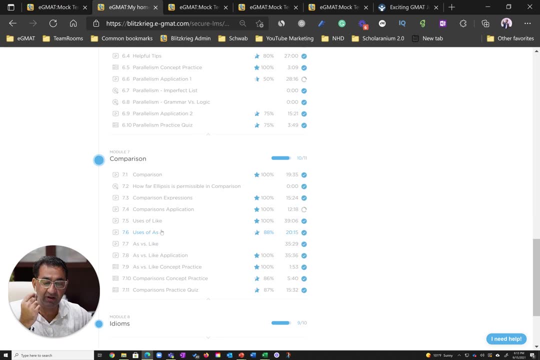 Let's kind of remove the filter here- And you can really see many other files where he spent a considerable amount of time as well. Again, this just shows that he wanted to excel. He wasn't just looking at finishing the course. You can see more evidence of the same in critical reasoning, where 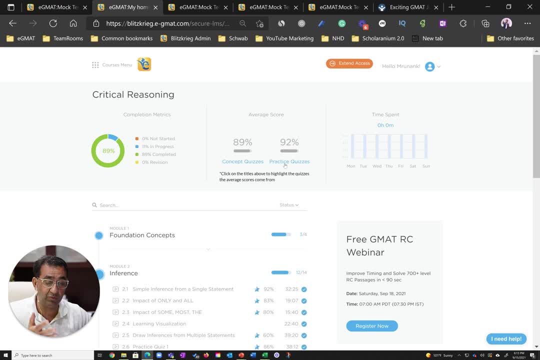 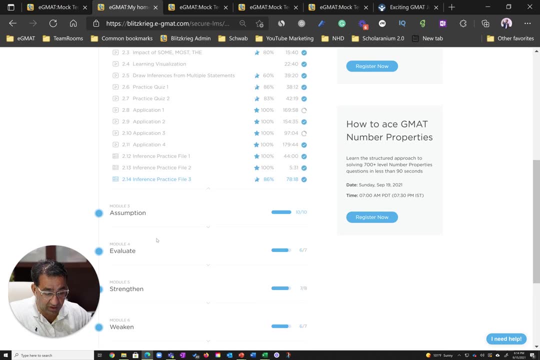 he didn't do many files in the first go, yet he revised, which is what led to these excellent scores. Examples of the same are about. you know, 170 minutes spent on application file one. Examples of the same also come up, So you can see that he spent a considerable amount of time on application file two, And so you can see that he spent a considerable amount of time on application file three, And so you can see that he spent a considerable amount of time on application file two, And so you can see that he spent a considerable amount of time on application file three And so. 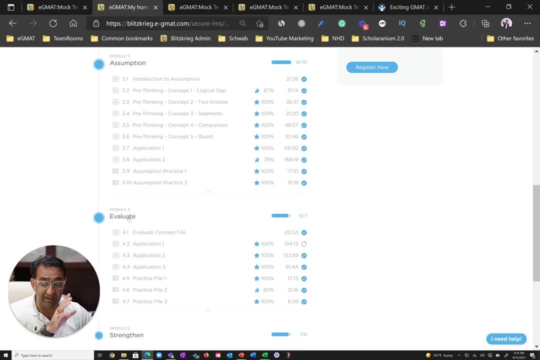 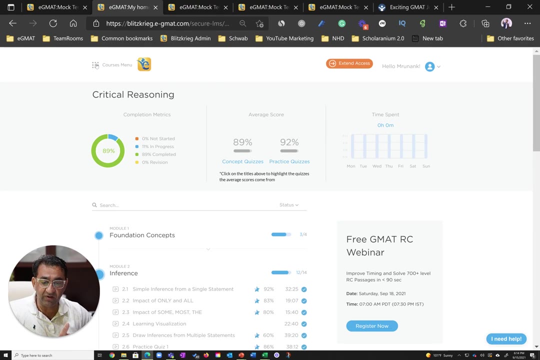 on and so forth. These are big courses. They require someone to stay focused for about 30 to 40 minutes, which is what the length of each activity is. The very fact that Ronan was able to do this, one after the other, shows that effort over there. Now, once he was done with these courses, 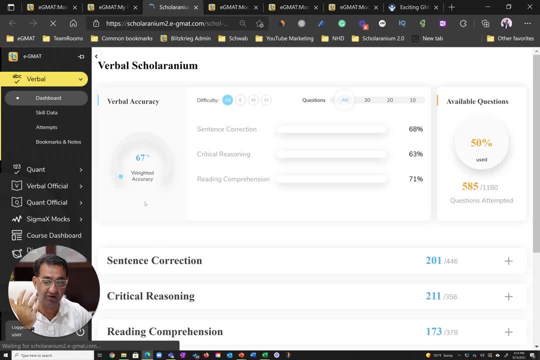 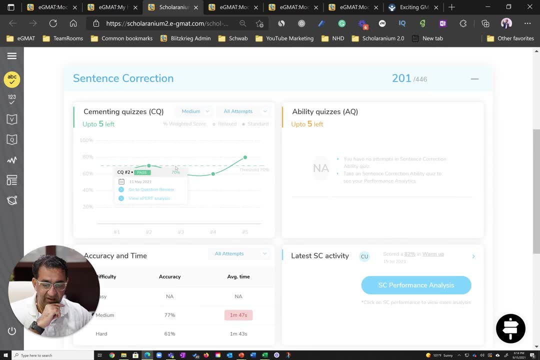 Ronan went and cemented his learning and which is where he leveraged our Scholaranium. Let's go into the sentence correction module. Well, let's actually expand that. You can see how he's gone through cementing quizzes. Again, there were quizzes where he did not score as well as he should have. He did the strategic review. 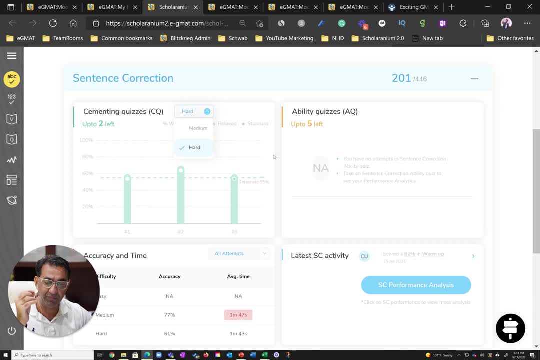 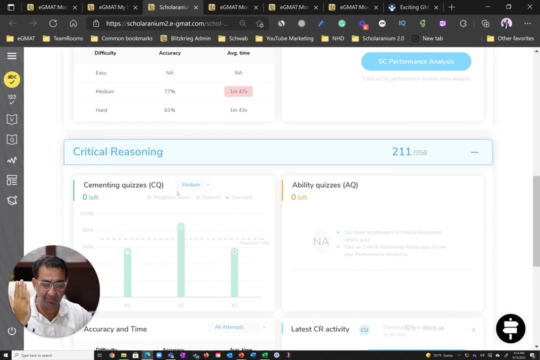 was able to get there. Then he moved on to hard quizzes and because he did well in medium cementing quizzes, he was able to score above the threshold in hard quizzes. You can see the same thing happen in critical reasoning, where he scored above the threshold of 70%, and hard cementing quiz is. 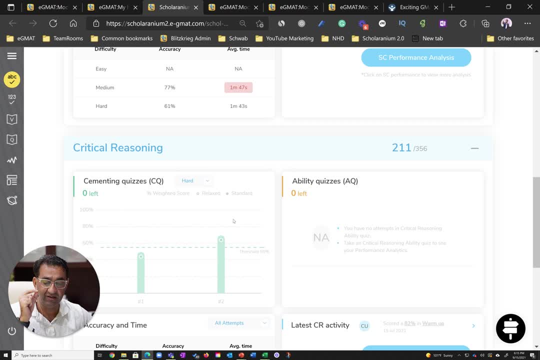 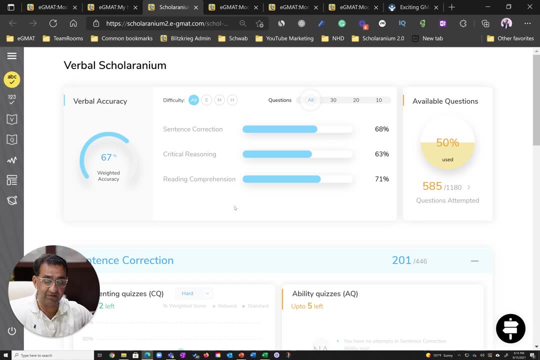 excellent. It's an indication of a 90th percentile student. Now, once he was done with cementing, Ronan went into test readiness. I'm going to actually show how he did test readiness, but because he did test readiness well, 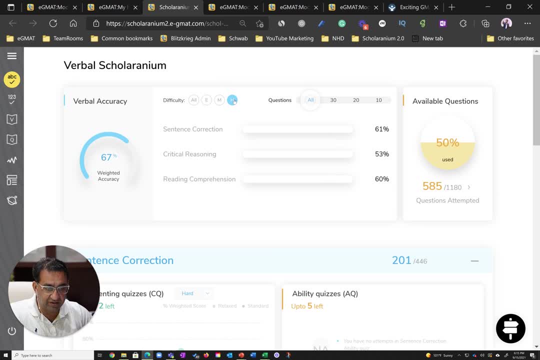 his metrics overall improved. You can see this When you look at his overall metrics. his hard metrics are good, but then in critical reasoning they're below threshold. In sentence correction they're just above threshold as well, as in RC as well. But if you take the filter to 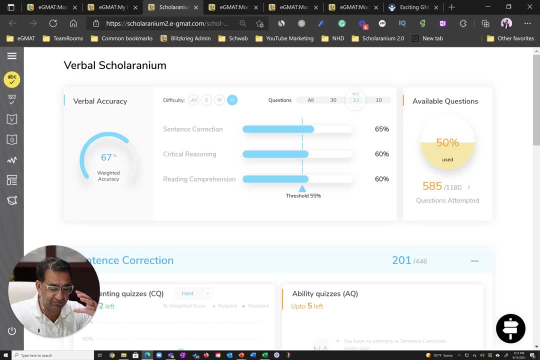 the last 20 questions, these metrics look a lot better. Now. this may seem incremental improvement, but in the context of the GMAT, this incremental improvement is huge. on hard questions, Not just that. on medium questions, Ronan was almost perfect You. 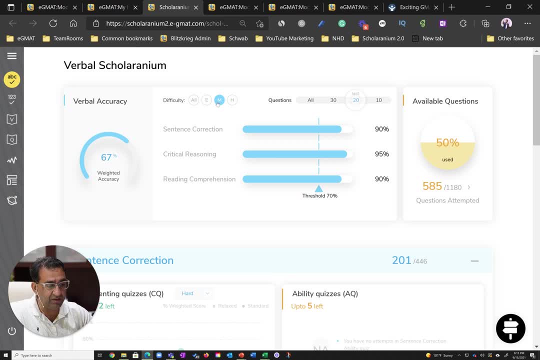 can see about 90% accuracy or higher in medium questions, which means on the actual test, Ronan went into the high ability zone right into the test. He got maximum opportunity to enhance or increase his scores, or so Now let's talk about the test readiness and how Ronan used it. 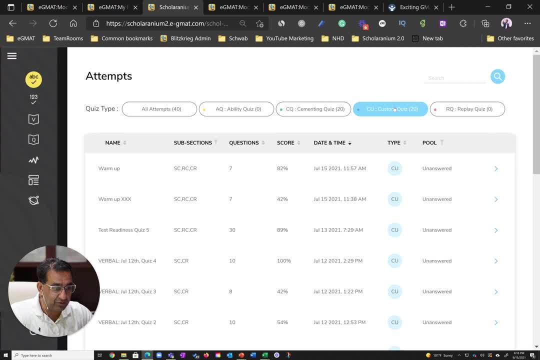 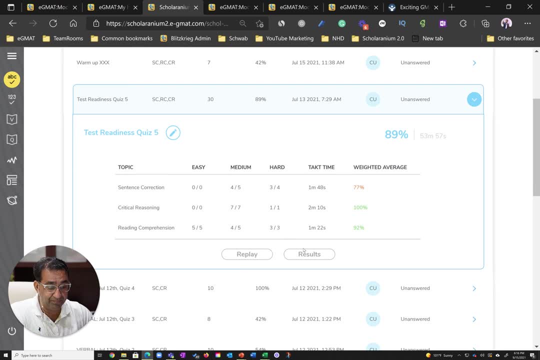 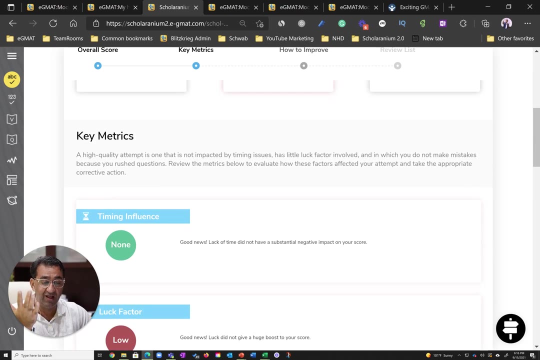 Ronan used data in test readiness. Ronan did about 20 test readiness quizzes. Now some of these test readiness quizzes were as big as a mock or so Now he did these quizzes He did really well. Despite that, Ronan spent a lot of time on improving these scores further. How did 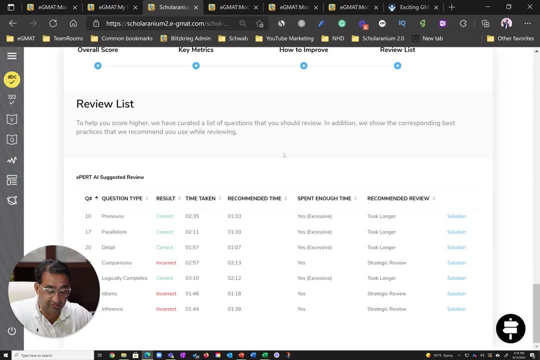 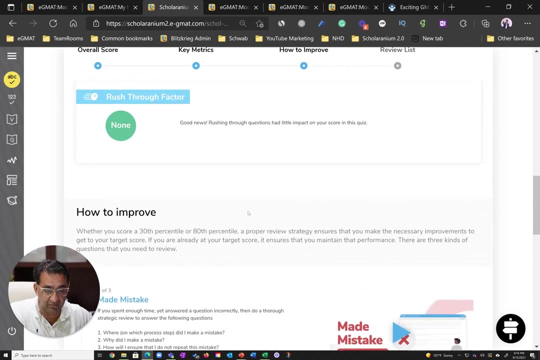 he do it. He looked at the review list that our AI generates, which not only looks at questions that you answered incorrectly, but questions that you've taken longer, or questions where you've that you probably made a mistake because you did not spend enough time, or so. 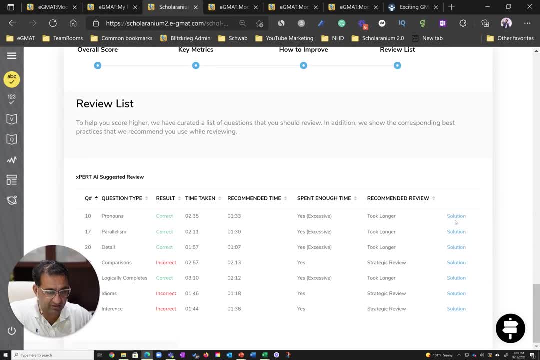 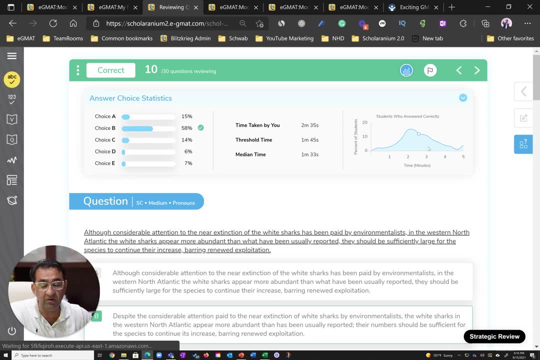 And by looking at those questions- and let's take a look at this question over here, where he took about two and a half minutes when he should have taken about a minute and a half- what this did was the system told him that he was in the 70th percentile. 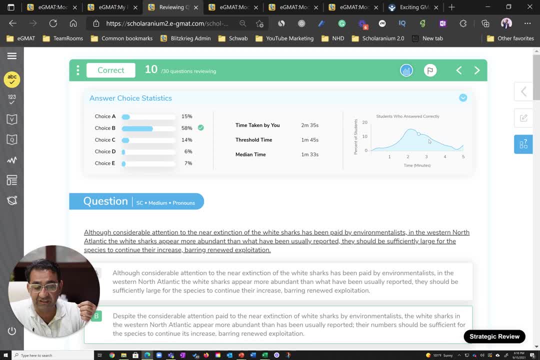 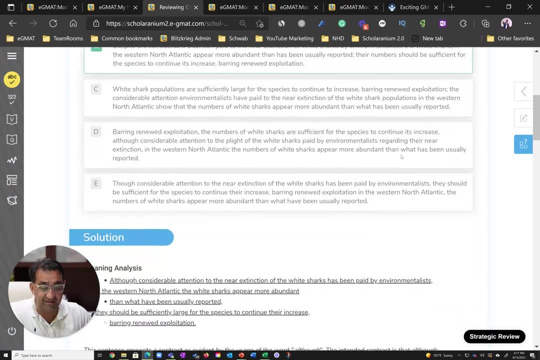 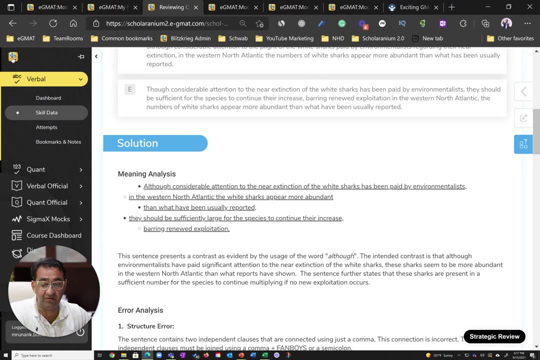 and even though he solved the question correctly, a question like this could potentially lead him to waste precious few seconds on the test. But revising that solution, the detailed solution here, he could then make sure that he gets to this question faster, or a similar question faster. 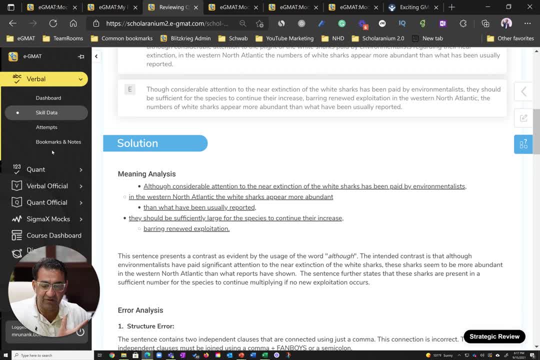 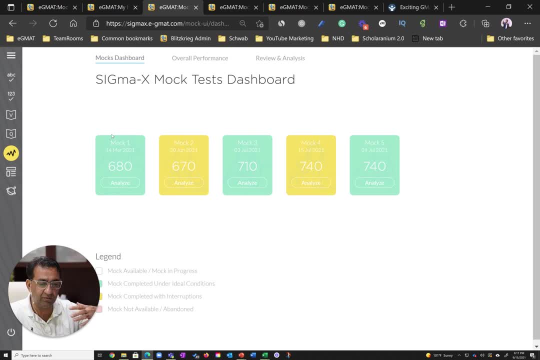 on the real test Now. when he did cementing and test readiness, he was then ready to take Sigma X mocks and you can see how his performance improved on the Sigma X mock, Starting from that 620, when he improved on his quant, he was able to get to a 680 in February and then to a 710 in. 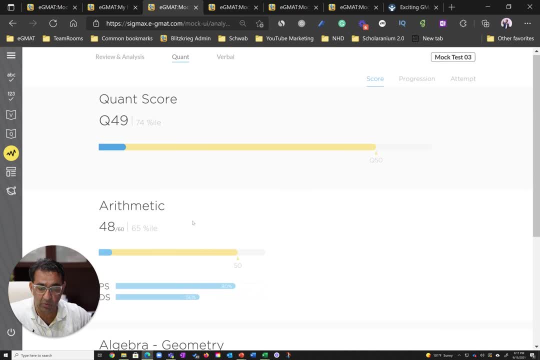 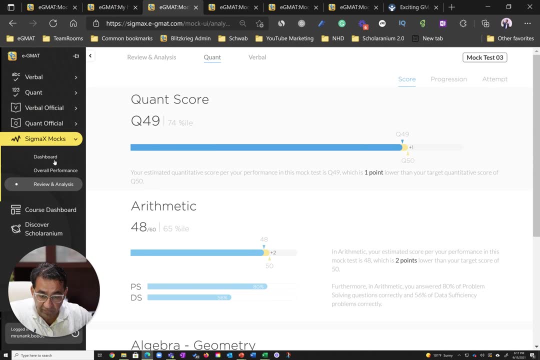 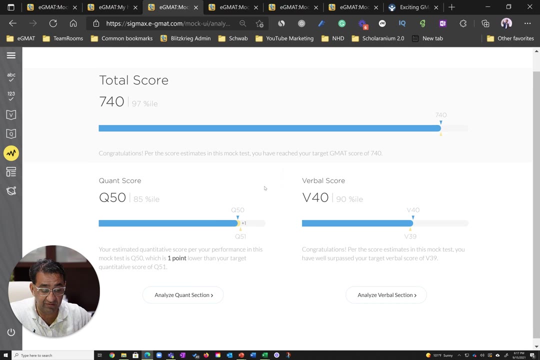 July where he had a good quant score and a really good verbal score. Within quant you can see that improvement. in algebra That's almost a perfect score. Now, once he furthered the test readiness, he was then in 20 days able to improve his score from a 710 to a 740.. You can see his ability scores in SC CR. 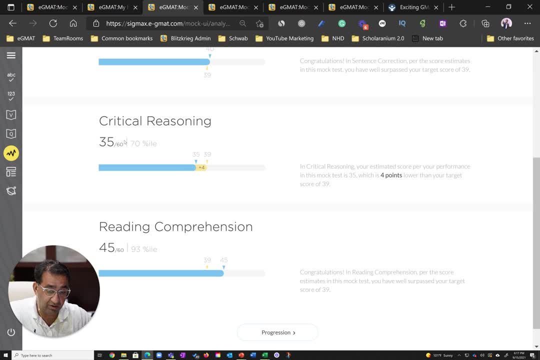 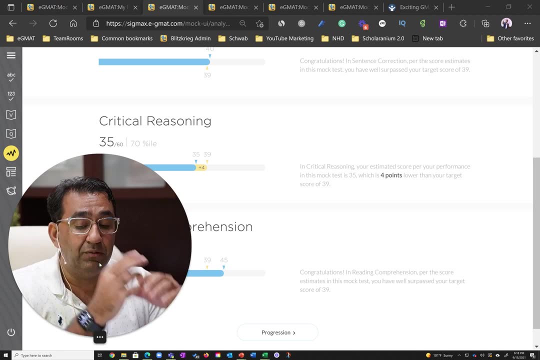 and RC, Really good ability in SC, great or good ability in CR, and while maintaining his excellent ability in reading comprehension. Now most people need about 150 hours to go from a 620 to a 740, or about 120 point improvement or so These 150 hours for most working professionals take. 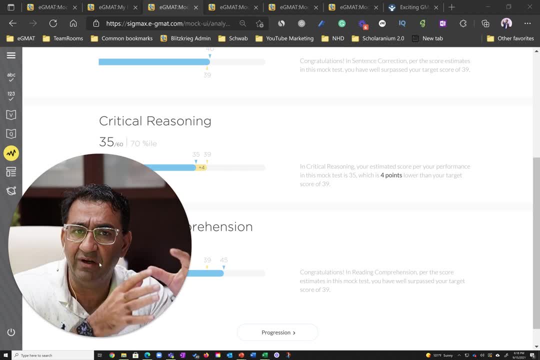 about two months. On the other hand, if you're looking for a 70 to 80 point improvement, you can do that in about a month if you devote about 20 hours a week learning for the GMAT. If you're seeking for a 120,, 150,, 200, or an 80 point improvement and you need a deterministic plan,